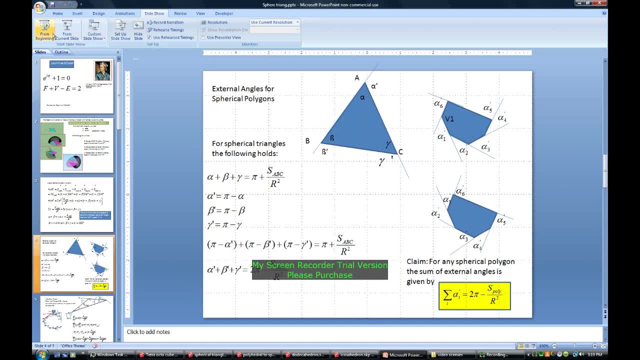 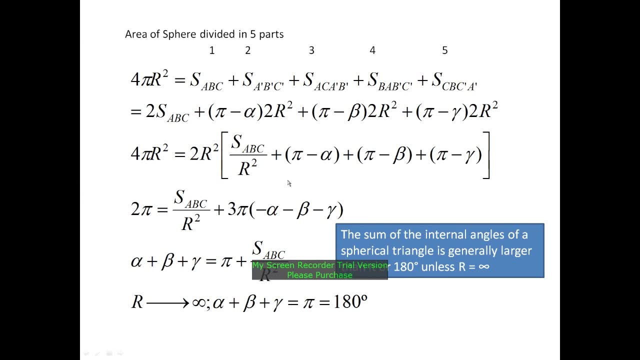 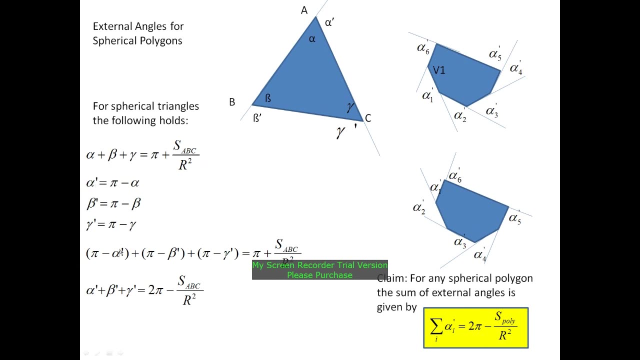 We see over r squared. we covered that, But there's more. we can look at it in terms of the external angles just by writing this equation, replacing alpha with pi minus alpha prime, alpha prime being pi minus alpha. So that's pretty symmetrical And we just get the sum of the external angles: is alpha prime plus beta prime. 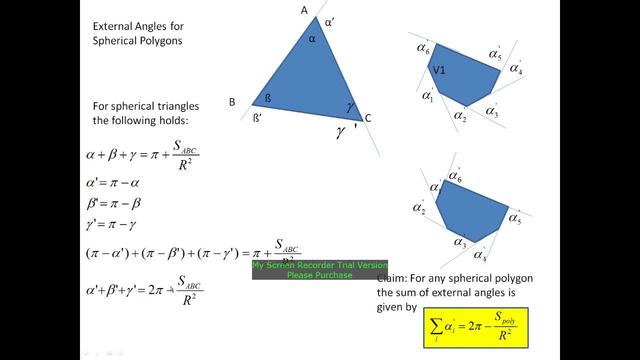 Plus gamma prime equals two pi minus the area sabc over r squared. Now, if you look at a more complicated than a triangle polygon, you see like as you add more vertices. generally speaking, the internal angles keep getting larger and larger and larger, But the external angles tend to get smaller and smaller and smaller. 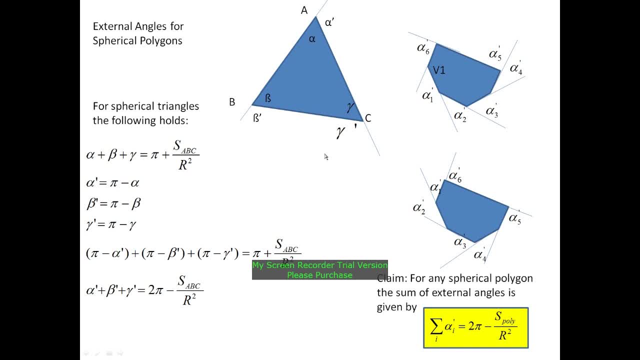 That really leads to a situation where the sum of the internal angles, since they're getting bigger and there's more of them, increases very rapidly, but the- at the very least we know- the sum of the external angles has to increase rather slowly. And here we make a claim that the sum of the external angles for any polygon is actually two pi minus the area of the polygon divided by r squared. 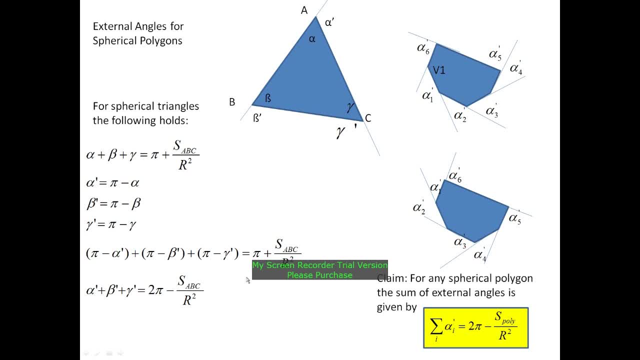 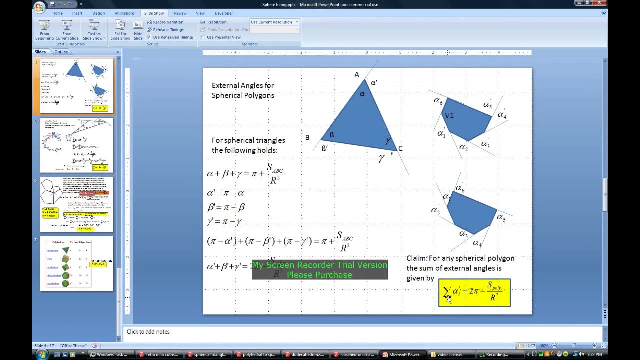 And so we'll just show that is true. Yeah, pretty remarkable fact. Certainly wouldn't be something true for a non-spherical coordinates, But let's look at what the proof of that might be. Okay, so let's look at whether we can prove this statement here, that 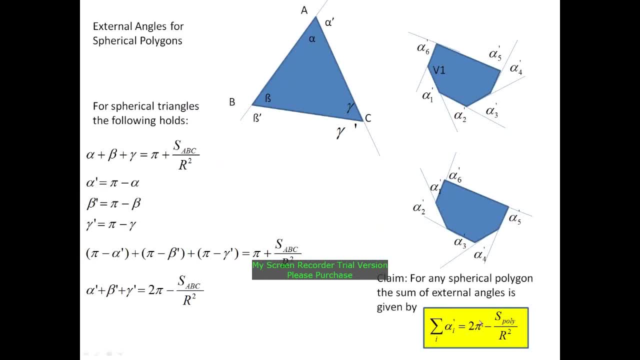 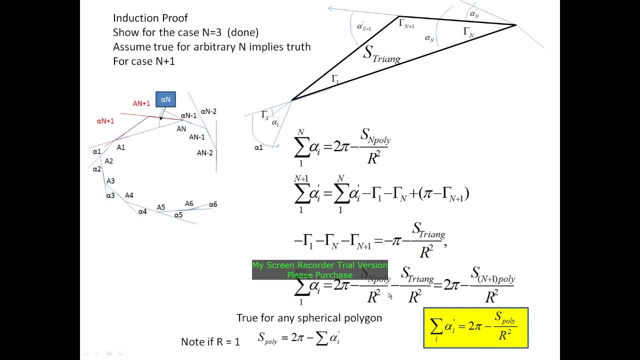 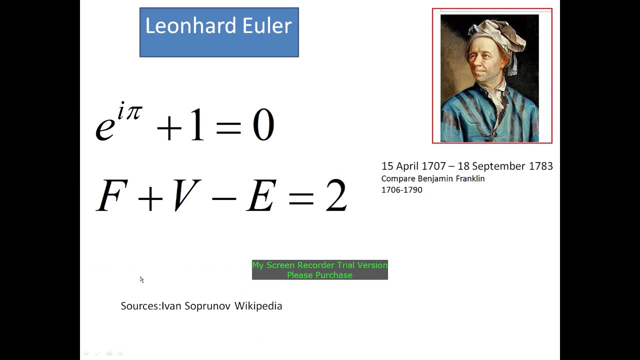 the sum of the external angles of any polygon, not just a triangle, is equal to two pi minus the area of the polygon divided by r squared. And the method for doing that will be- and I just want to give credit to the proof I'm following here is by this guy, Ivan Sopranoff. I think he's a professor at Cleveland State University or someplace. 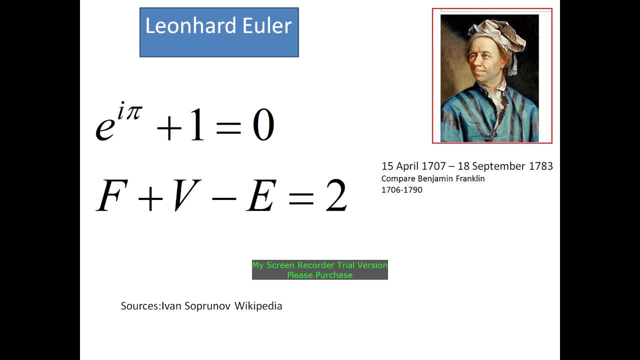 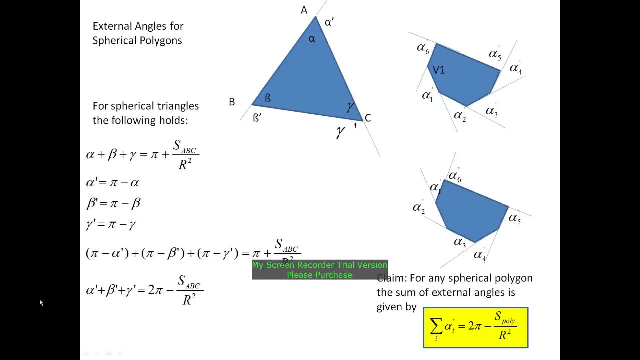 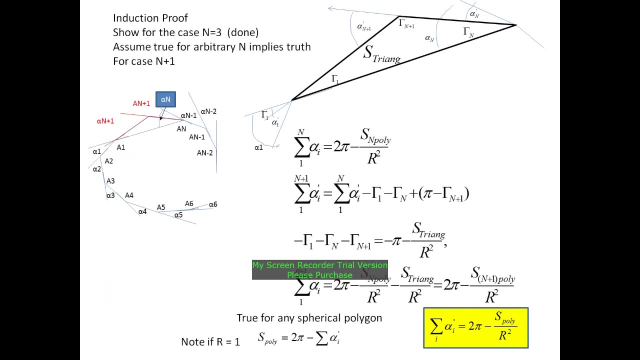 Anyway, you can look up spherical triangles or Euler And Sopranoff. you'll come up with his publication and I'm sort of following that publication. I just don't want to. all I'm taking credit for is the sketchup artwork in my own befuddled explanation here. 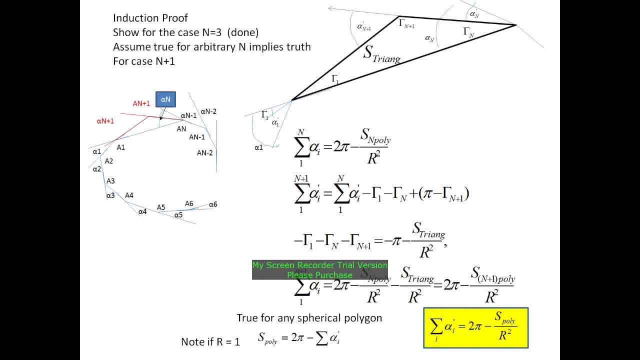 So how do you prove this for the general polynomial, I mean general polygon. Well, first you show it's sort of a modified version of an induction proof. Show it for the case where the number of vertices is equal to the number of vertices divided by r squared. Well, first you show it's sort of a modified version of an induction proof. Show it for the case where the number of vertices is equal to the number of vertices divided by r squared. Well, first you show it's sort of a modified version of an induction proof. Show it for the case where the number of vertices is equal to the number of vertices divided by r squared. 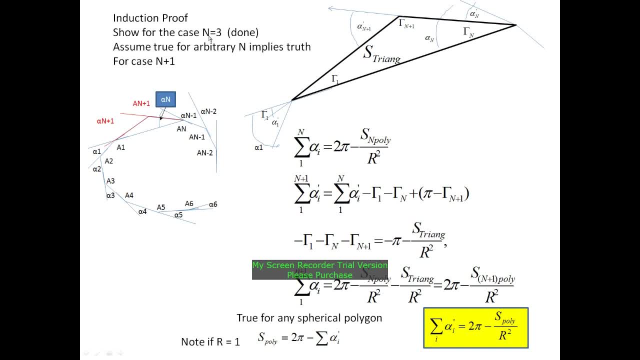 where the number of vertices equals n equals 3, that we've already done. that's the triangle. For any triangle, the sum of those angles is 2 pi minus s-poly over r-square. Then assume it's true for some arbitrary n, or assume the truth for some arbitrary n. 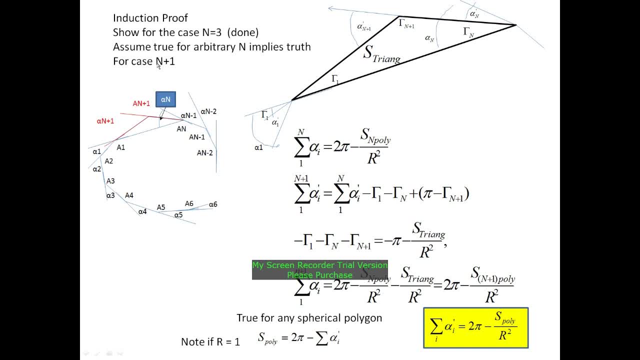 implies truth for the case n plus 1.. That means show basically that if it's true for 3,, it'll be true for 4.. If it's true for 4, it'll be true for 5, and true for 6, and so on for all the finite numbers. 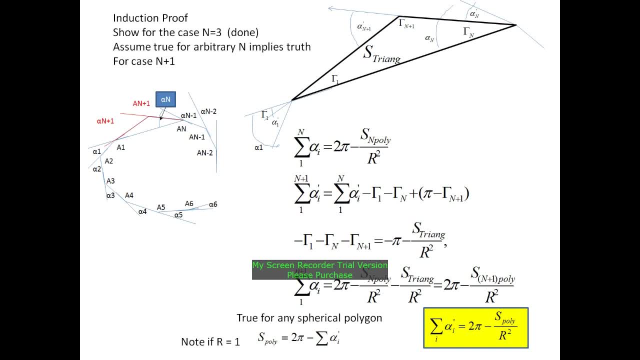 So, for arbitrary n, assume it's true and show that you can use that assumption to prove the n plus 1 case. Okay, some of the- and I'm just going to leave out the primes here because it's just easier- 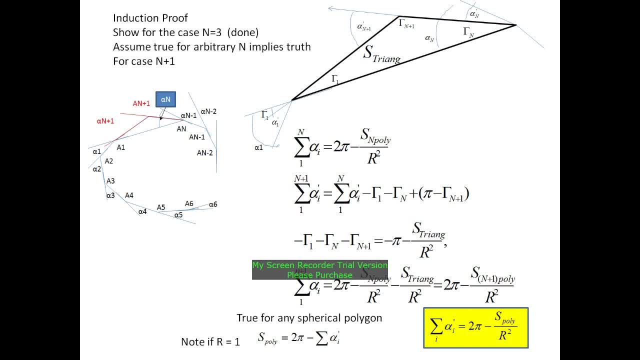 I wrote that in PowerPoint. It's just easier to keep it that way. Okay, sum of the- assume it's true that the sum for an n. so here we just draw a representation. This is pretty much Sopranoff's figure. that's why I'm trying to give him credit for it. 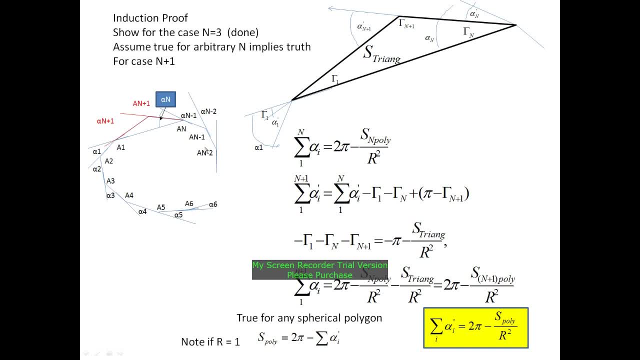 So you draw this arbitrary figure here that shows an arbitrary polygon of n vertices, and then you add one more vertex to it, the a, n plus 1, and you see what happens. So for the n polygon you assume the relationship is true. 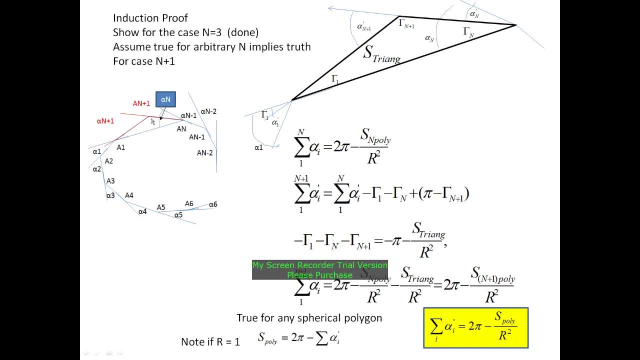 Then what changes when you add the extra polygon? Well, you get a larger area, and that area is this triangular region, and the vertex of that triangle, of the added region, will be a vertex at a- 1, a vertex at a n plus 1, and a vertex at a n. 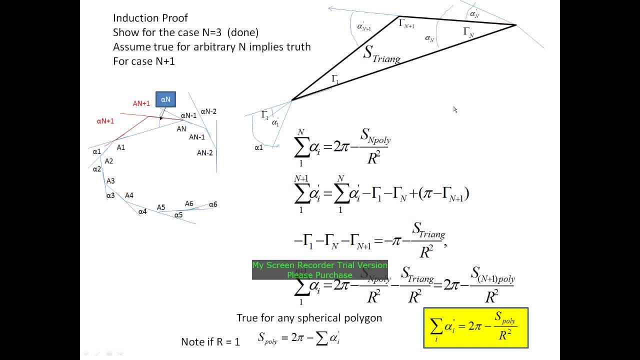 I just drew a larger version of it here. So basically most of the external angles going around the polygon are exactly the same. So when you want to solve for this thing, that you want to demonstrate the sum of alpha prime i from i 1 to n plus 1,, 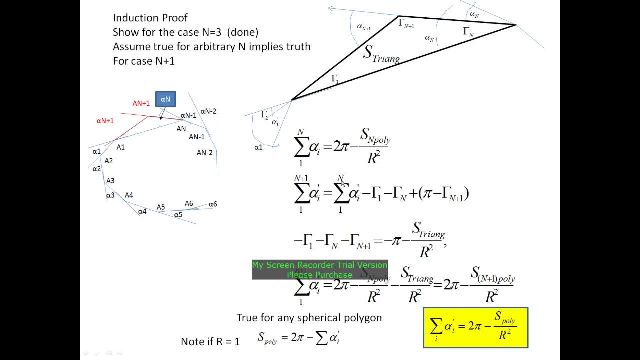 it's basically the same as the alpha primes from 1 to n, except for at vertex a n, vertex a, 1, and vertex a n plus 1.. So, and the difference is, here's the angle, external angle, at a, at vertex n. 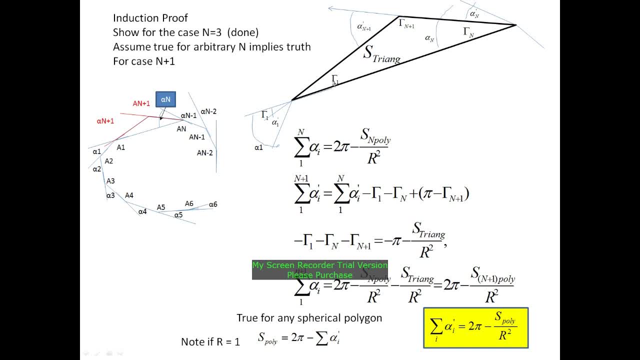 What you did is subtract off. I called the internal angles here gamma 1, gamma n and gamma n plus 1.. So to get the new external angle, external angle at n plus at n, you just subtract off gamma n. The same thing here to get the 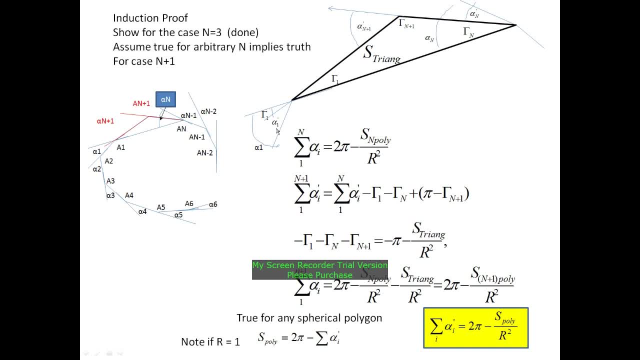 new external angle at vertex 1, a1, you just subtract off gamma 1.. And then you have the new external angle alpha prime n plus 1.. So that's what I'm showing here In terms of gamma 1, gamma n and gamma n plus 1, the sum of external angles for the n plus 1 case. 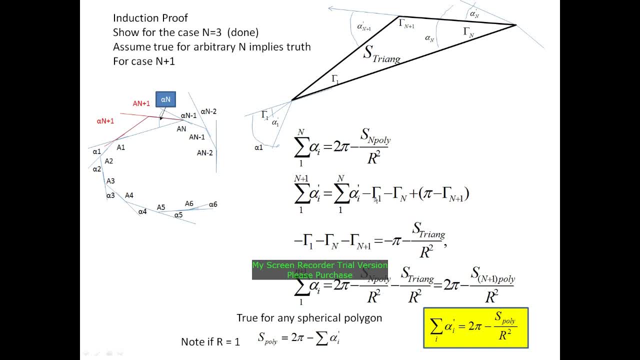 is just the sum for the n case minus gamma 1, minus gamma n and minus gamma n plus 1.. And then plus pi. Okay, So if we want to solve, we can get an expression for this. This is just minus what we started out here with. 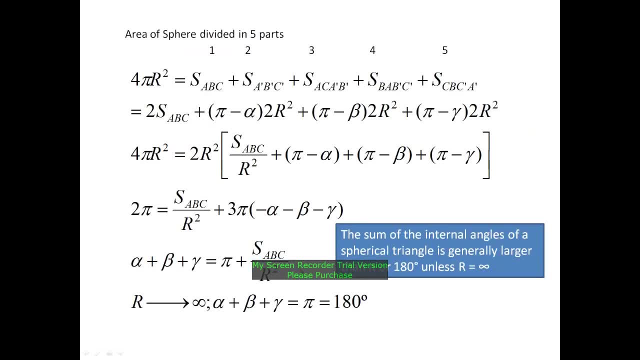 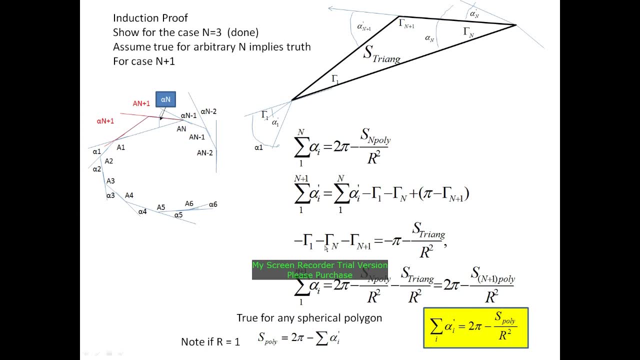 That's just minus pi, minus gamma 1, minus gamma n, minus gamma n plus 1.. That's what we showed in the beginning. It's just minus pi, minus the area of this new triangle that we added on, divided by r squared. So we replace gamma 1, gamma n, gamma n plus 1, those random. 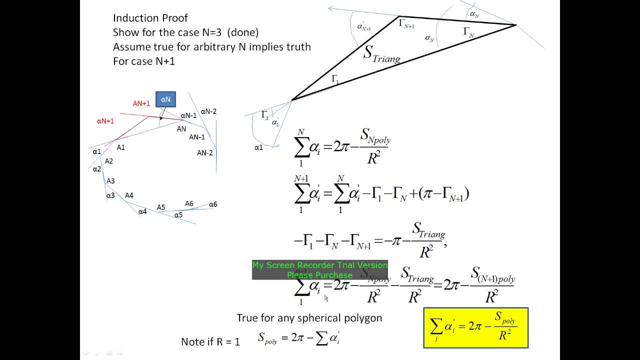 angles With this expression. so we end up getting 2 pi minus the area of the n polygon over r squared, minus the area of the triangle over r squared, And that just equals 2 pi minus the area of the n plus 1 polygon divided by r squared. So that's what we needed to. 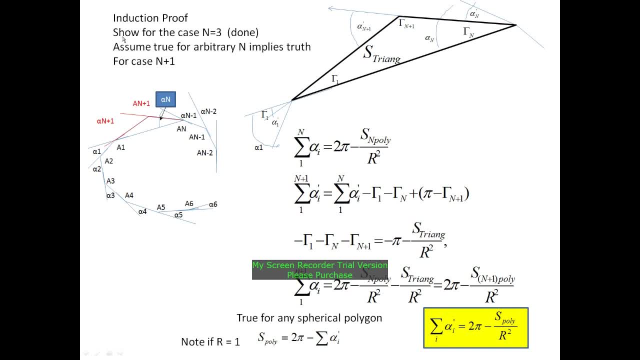 prove to solve the problem. So we're going to use the induction criterion. So if it's true for n, it's true for n plus 1.. Since it's true for 3, it's true for 4,, 5,, 6,, 7, any n. So in general, for any spherical. 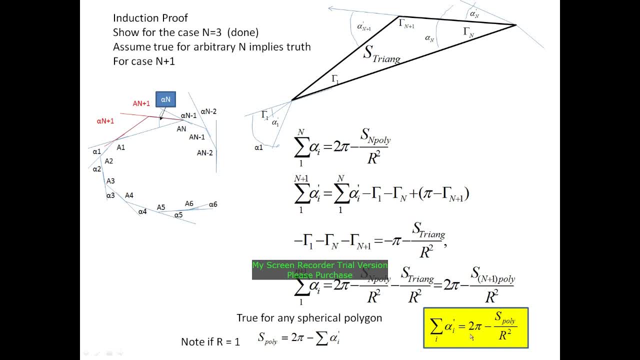 polygon. we can now say that the sum of the external angles is 2 pi minus the area of the polygon divided by r squared. And just as a note, we're going to use this in the next part. So if r, if it's a unit sphere- a lot of times people work with unit spheres and spherical. 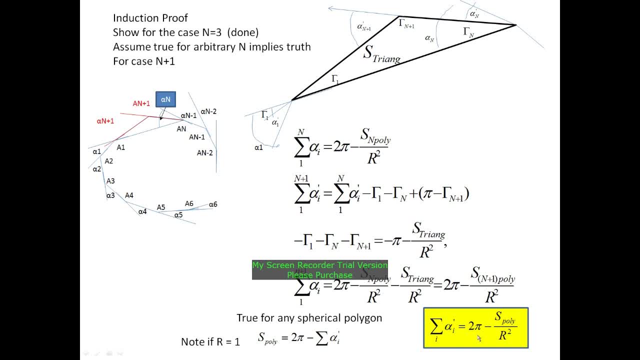 trigonometry, just so you can drop out the r, then the area you can solve for the area of the polygon. The area of any polygon on a unit sphere is 2 pi minus the sum of the external angles of that polygon. So that's a pretty amazing result already. 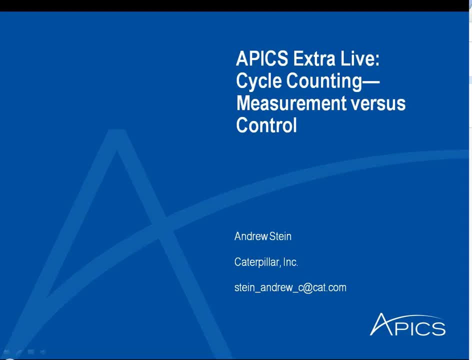 Hello and welcome to Apix Extra Live Cycle Counting, Measurement vs Control with Andrew Stein. My name's Christopher Jablonski, staff editor with Apix. Before we begin, I'd like to run through a few details At the end of the presentation.